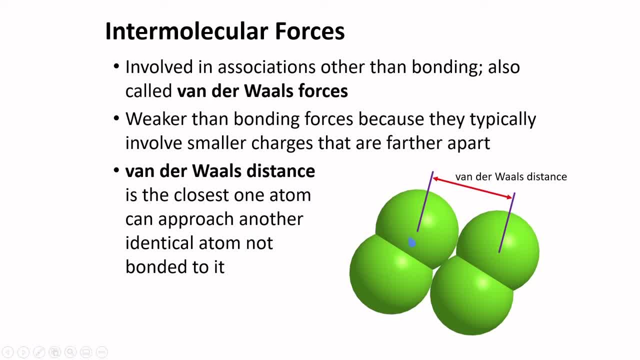 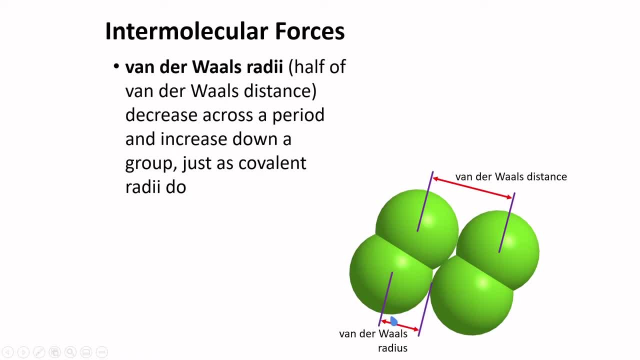 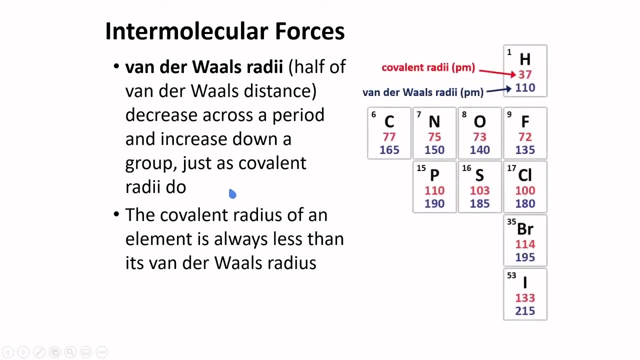 not bonded to it. as shown here, Van der Waals radii or half of the Van der Waals distance decrease across a therion and increase down a group just as covalent radii do. The covalent radius of an element is always less than its Van der Waals radius. 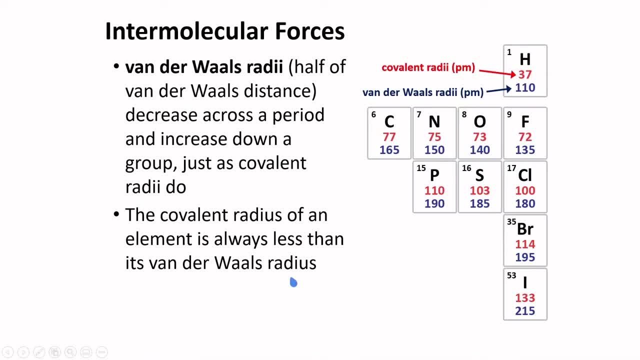 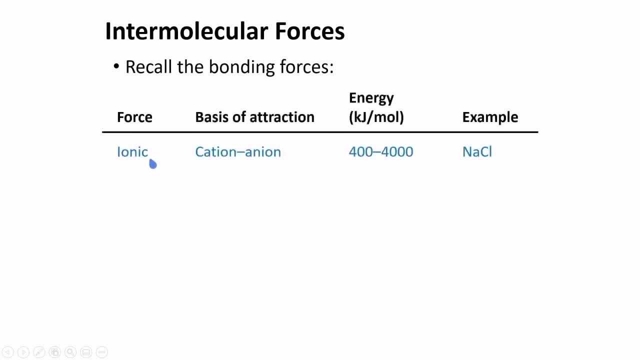 The covalent radius of an element is always less than its Van der Waals radius. The covalent radius of an element is always less than its Van der Waals radius. Recall the bonding forces. We have the ionic bonds. This is the attraction of a cation and anion. 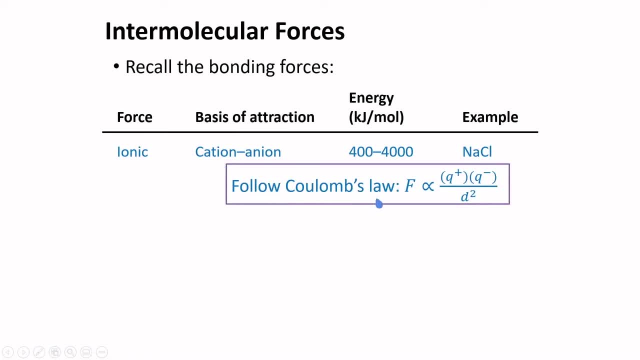 Here, what is important is the Coulomb's law, wherein the force of attraction is directly proportional to the charges of the particles and inversely proportional to the distance between them. Here, what is important is the Coulomb's law, wherein the force of attraction is directly proportional to the charges of the particles and inversely proportional to the distance between them. 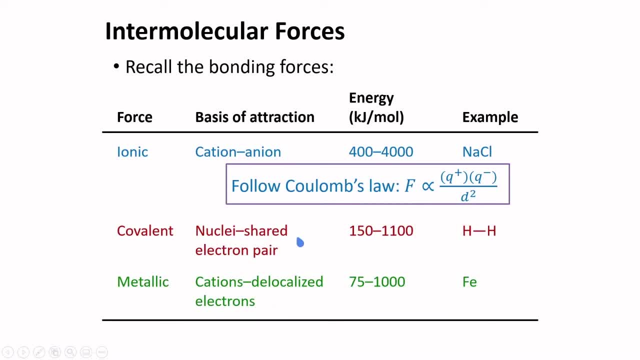 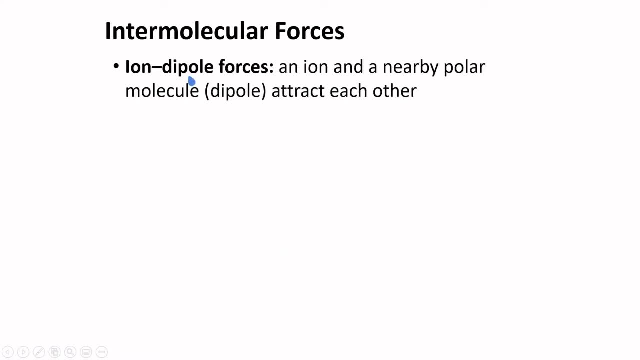 Covalent bonding involves the nuclei and the shared electron pairs, And metallic bonding have cations and the localized electrons. And metallic bonding have cations and the localized electrons. The first type of intermolecular forces is ion-dipole forces. This is formed by an ion and a nearby polar molecule. 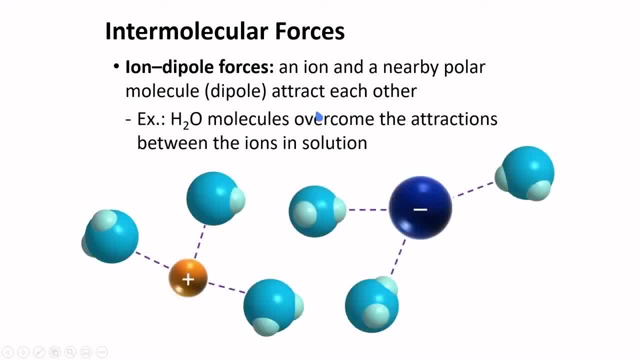 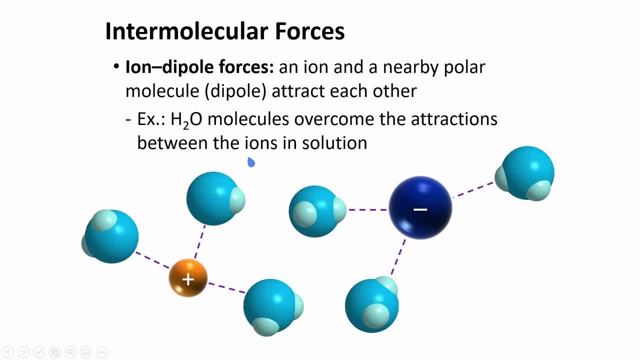 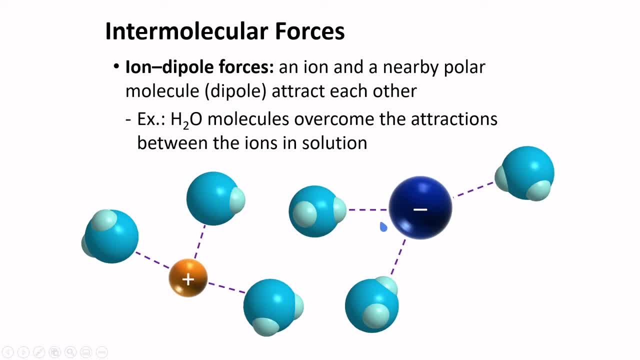 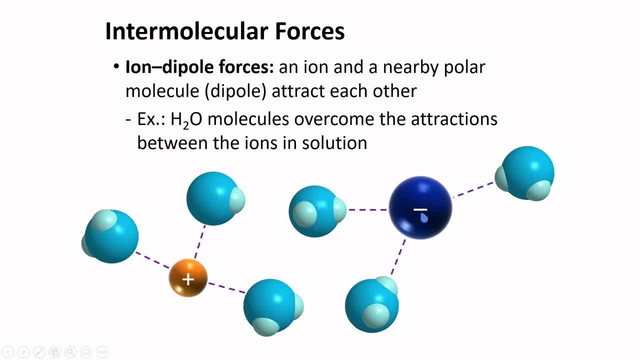 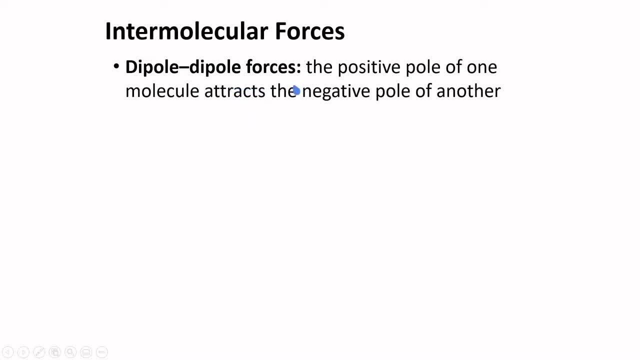 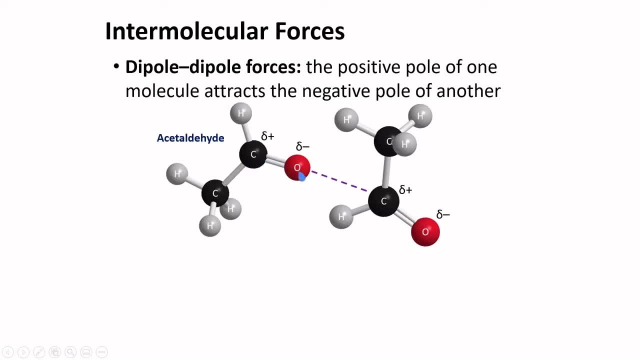 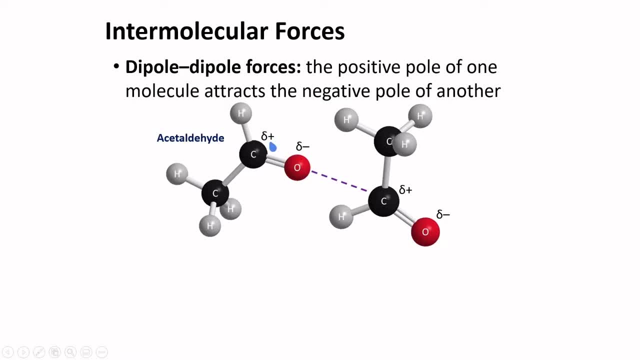 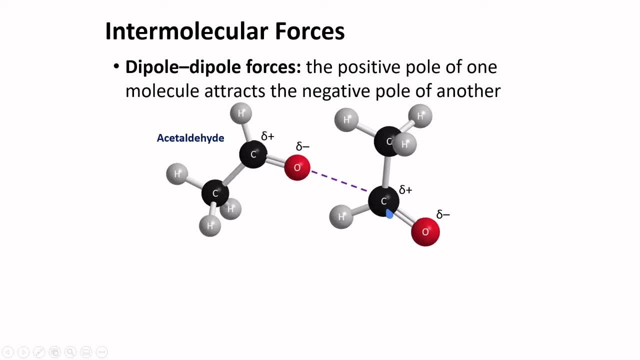 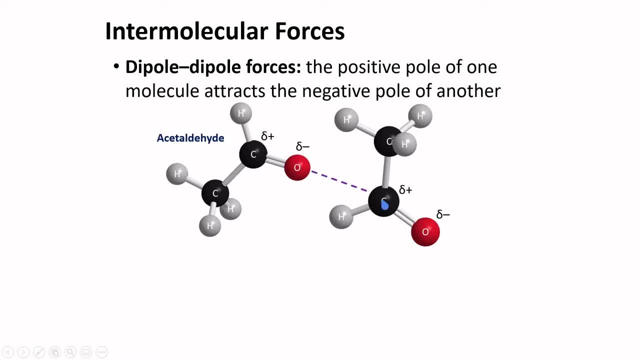 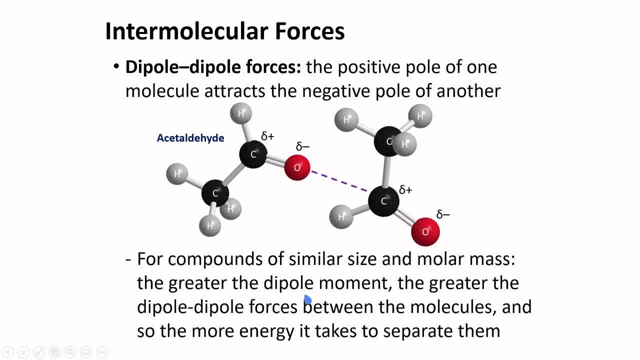 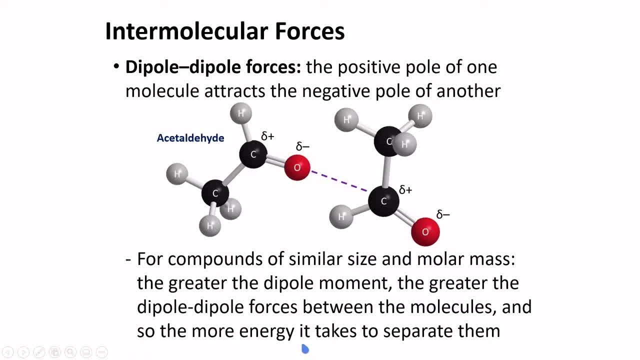 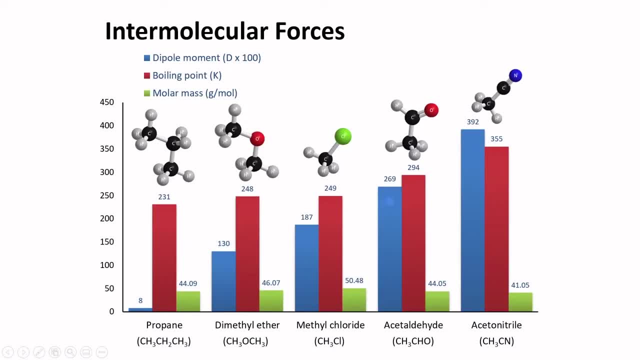 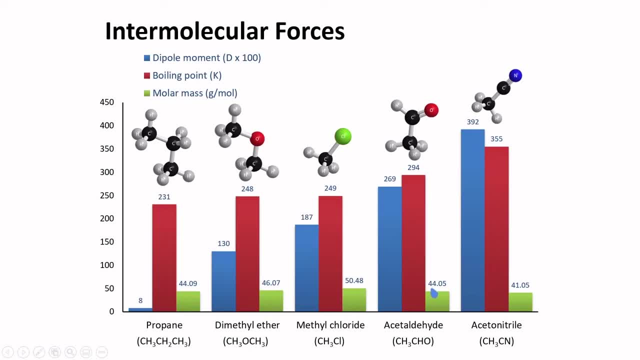 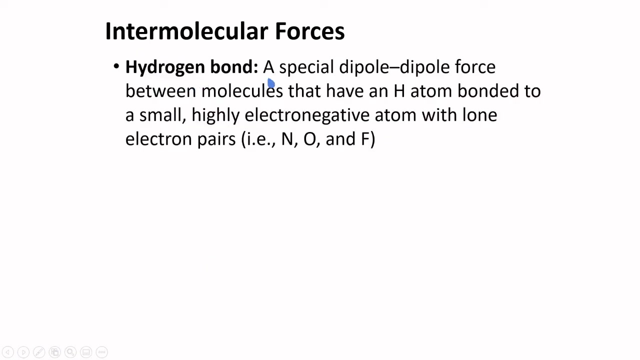 Take note that these molecules have nearly the same molar masses. thus higher dipole moment translates to higher melting and boiling points. Hydrogen bond is a special dipole-dipole force between molecules that have a hydrogen atom bonded to a small, highly electronegative atom with lone electron pairs. 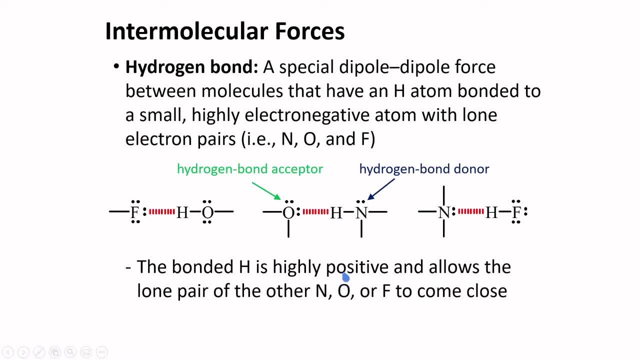 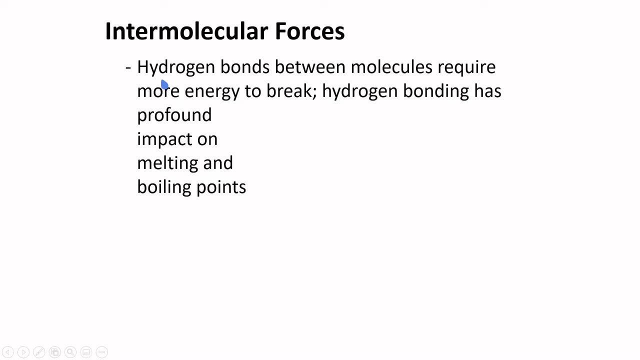 The bonded hydrogen is highly positive because of the electronegative atom bonded to it and allows the lone pair of the other, nitrogen, oxygen or fluorine, to come close. Take note that hydrogen bonding only occurs on these situations. Hydrogen bonds between molecules require more energy to break. 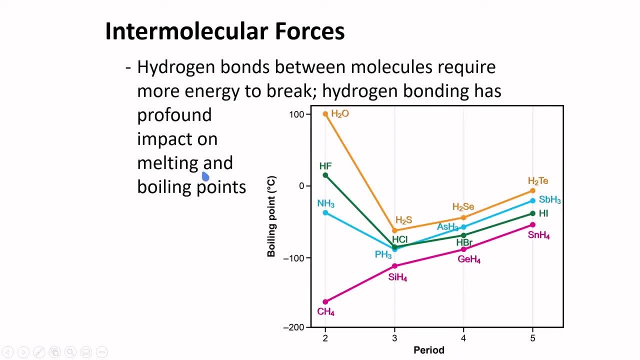 Hydrogen bonding has profound impact on melting and boiling points. In the splat of boiling points With atoms of the same groups bonded to hydrogen, you will notice a downtrend from H2Te, H2Se and H2S. We can say the same thing for HI, HBr, HCl. 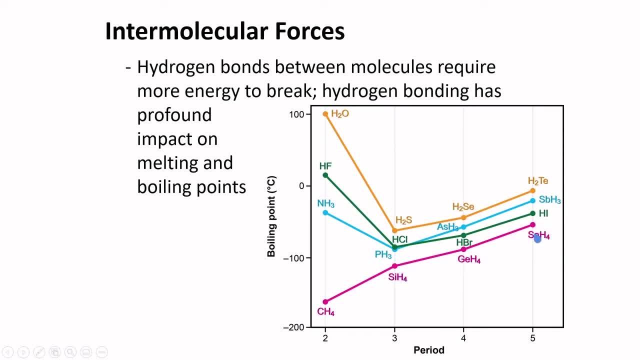 In fact, in the case of Stannane, Germaine, Silane and Methane, HCl and HCl are the same. In fact, in the case of Stannane, Germaine, Silane and Methane are the same. In fact, in the case of Stannane, Germaine, Silane and Methane are the same. In fact, in the case of Stannane, Germaine, Silane and Methane are the same. There is an obvious trend. 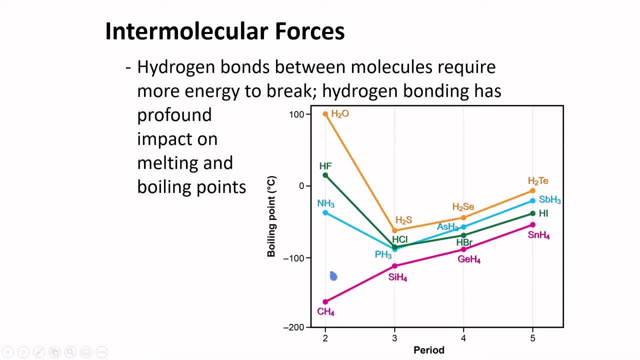 However, the hydrogen bonding breaks the trend and water has a very high boiling point. If we are to extrapolate this boiling trend, water should have boiling point at this level, And yet hydrogen bonding allows water to exhibit a higher boiling point. We can say the same thing for hydrogen fluoride and ammonia. 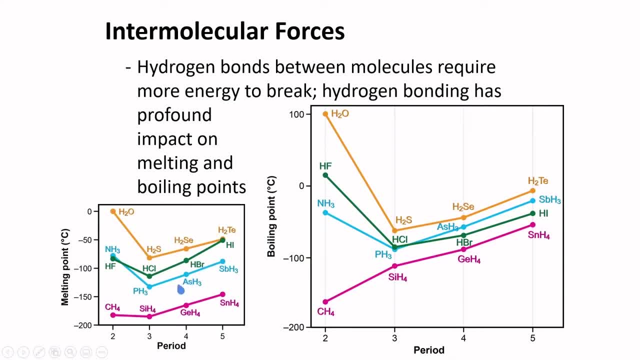 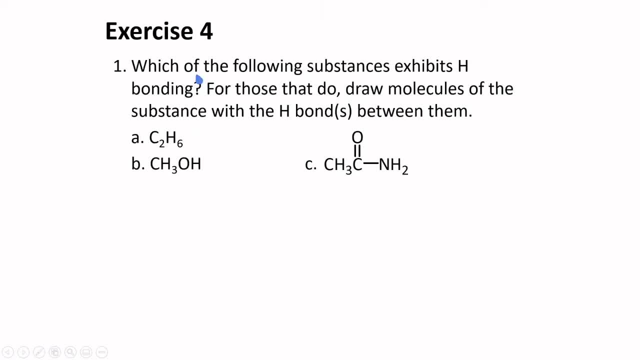 When melting points are compared, the trends are very similar. Which of the following substances exhibits hydrogen bonding? For those that do draw molecules of the substance with the hydrogen bonds between them, Letter A is ethane. The molecular structure of ethane is this one: 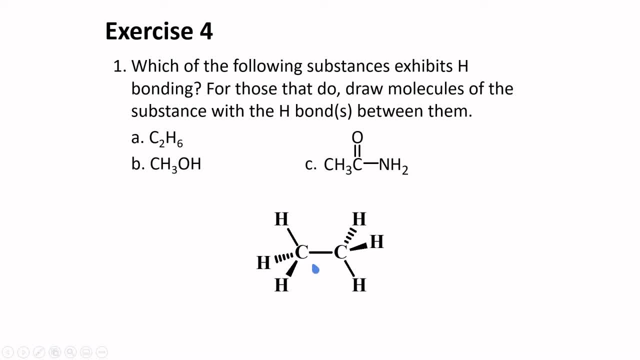 There are no oxygen, nitrogen or fluorine present. Therefore it does not exhibit hydrogen bonding. Letter B is methanol. Here a hydrogen is bonded to the oxygen. Hydrogen bonding is possible in this substance In the presence of another molecule of methanol, the oxygen, the hydrogen, and the oxygen in 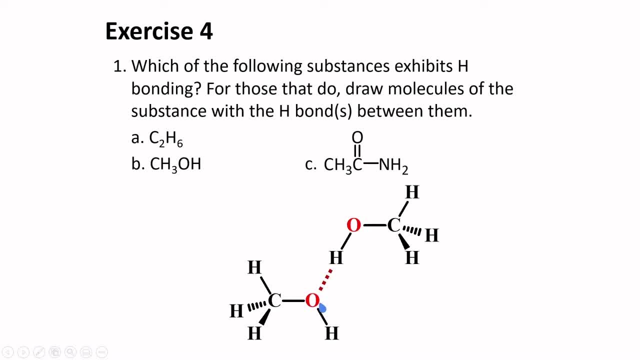 another molecule can form hydrogen bonding. Thanks for watching. See you next video Later. Bye. C is acetamide. In acetamide there's oxygen and nitrogen present. Hence hydrogen bonding can occur with this substance. The hydrogen bonded to nitrogen in one molecule of acetamide can form hydrogen bond with the oxygen. 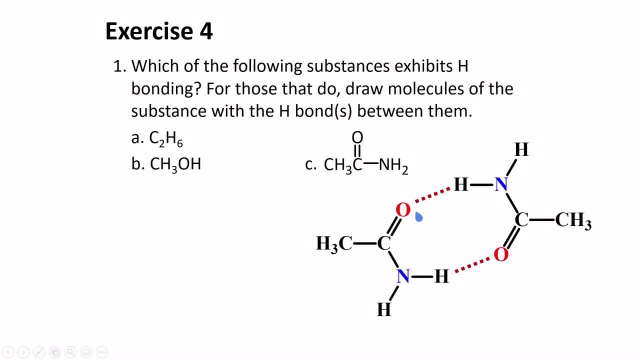 of another. Another hydrogen bond is possible when the hydrogen bonded to the nitrogen in acetamide forms a hydrogen bond with the nitrogen in another acetamide molecule. Explain the melting points of the following. We can compare the melting point of this compound to the melting point of this compound Here. the melting point is 388. 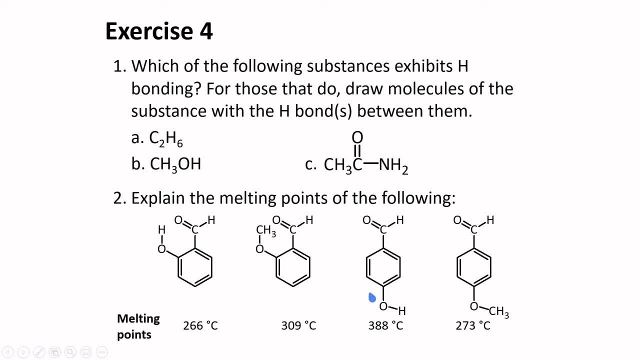 degrees Celsius, and this melting point can be attributed to hydrogen bonding. Now, why is the melting point of this substance lower than the melting point of this one? Here, internal hydrogen bonding can occur. This oxygen and this hydrogen can form an intramolecular hydrogen bond: Intramolecular hydrogen. 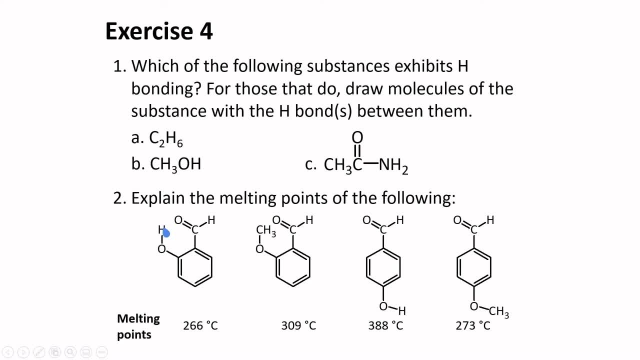 band tends to limit the inter molecular hydrogen bonding between molecules which has a large effect on melting points- Here intermolecular hydrogen bonding. tipping can happen in new informative when be found between the the different molecules of a closely linked Queensborough hydrogen band, Here intermolecular hydrogen bonding. immunity between molecules which has a large effect on melting point, Here intermolecular hydrogen bonding to that melting point. 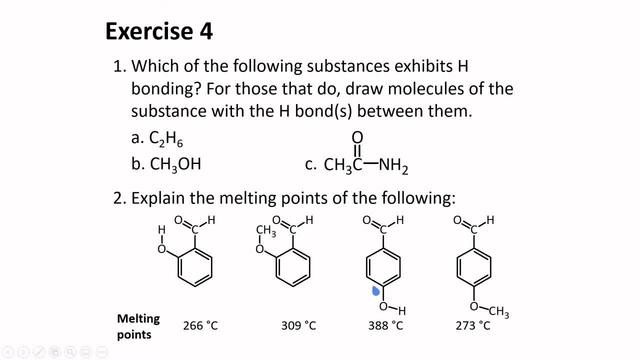 Here lipid new valve volume, even white offended vardı To wine also. in the benchmark of the correlation between Sacrum Antoni and C is a little bit different. molecular hydrogen bonding can occur quite easily, and so the melting point here is quite large. 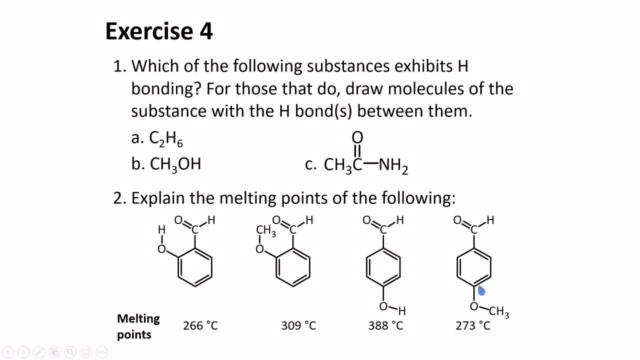 what about these two compounds? this compound has two oxygen atoms and they are present at opposite ends of the molecule. this arrangement enables the partial cancellation of band dipoles within the molecule. in this other compound, the oxygen are on the same side of the molecule and thus in this case dipole moment is oriented. 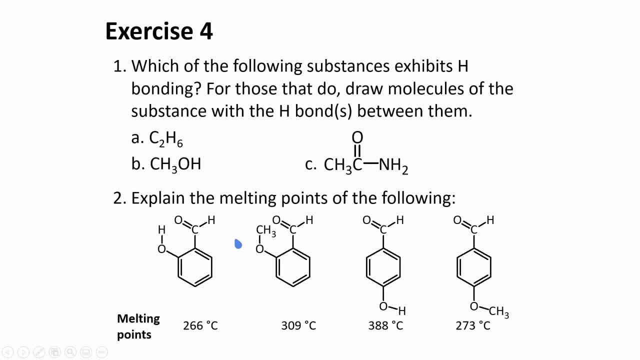 at this direction. as a result of the higher dipole moment expected for this compound, it has a higher melting point compared to this one. the higher melting point of this compound compared to this compound can be attributed to the larger molar mass and the higher dispersion forces that are present. 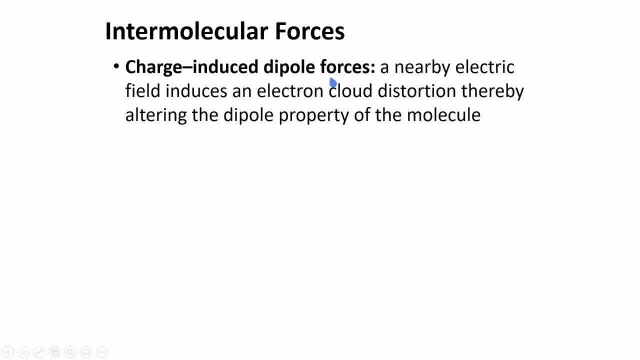 in charge induced dipole forces. a nearby electric field induces a electron cloud distortion, thereby altering the dipole property of the molecule. take note that the ease with which the electron cloud can be distorted is called its polarizability. for example, in the presence of a dipole, a non-polar substance can be polarized. 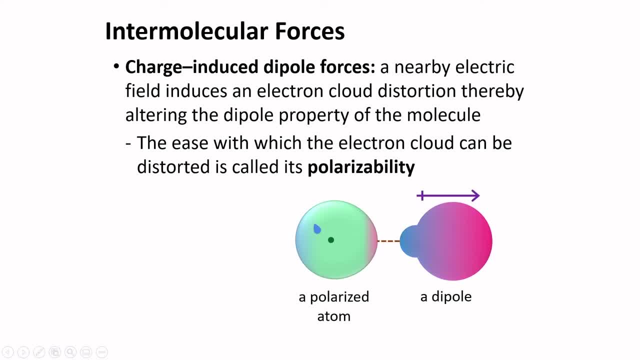 and induced to have a dipole property in the form of an ion. smaller atoms or ions are less polarizable than larger ones, and ions being bigger are more polarizable than their parent atoms. how about cations? cations are smaller than their parent atoms and they are less polarizable than larger ones. 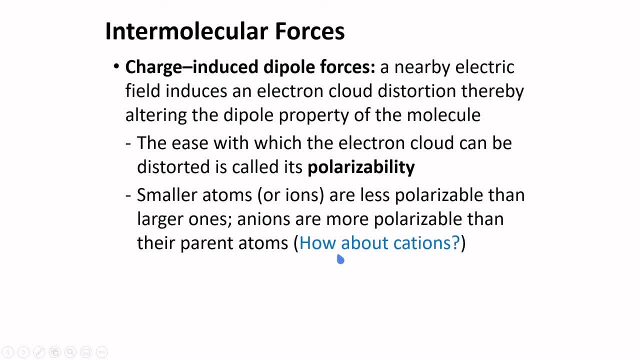 hence cations should be less polarizable. there are two types of charge-induced dipole forces. one is ion-induced dipole forces, wherein the electric field comes from the ion, and the other is dipole-induced dipole forces, wherein the electric field comes from a dipole. 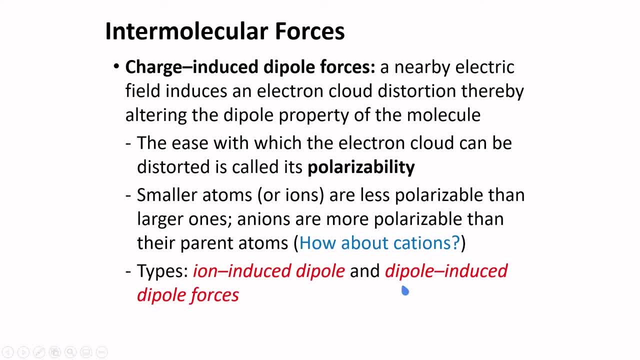 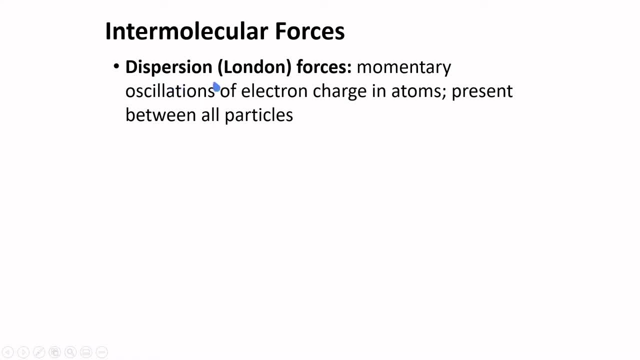 the last type of intermolecular forces are dispersion forces or London forces. these are momentary oscillations of electron charge in atoms and present between all particles. instantaneous dipole results from non-uniform distribution of electrons at an angle of the dipole and at an angle of the dipole. 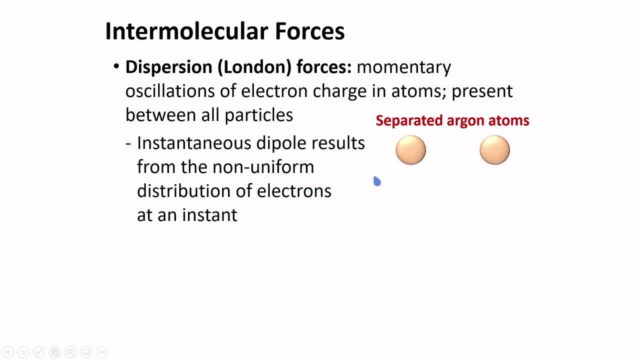 at an instant separated argon atoms can form dipoles. we call them instantaneous dipoles. as they come close to each other, the instantaneous dipole in one atom or molecule can induce a dipole in its neighbor. hence attraction can result even in non-polar substances. 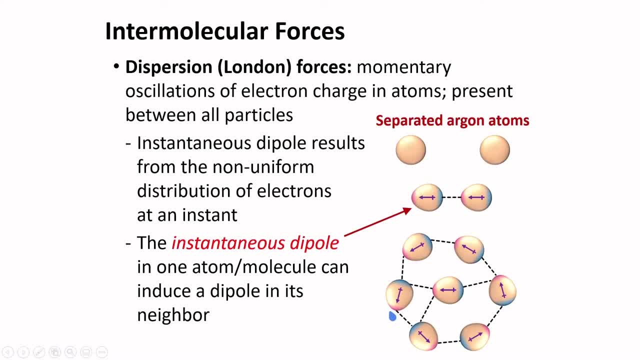 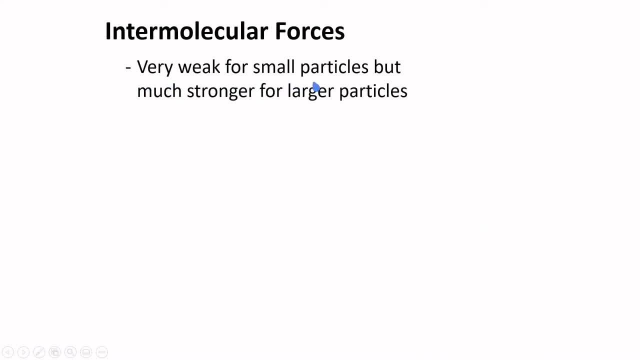 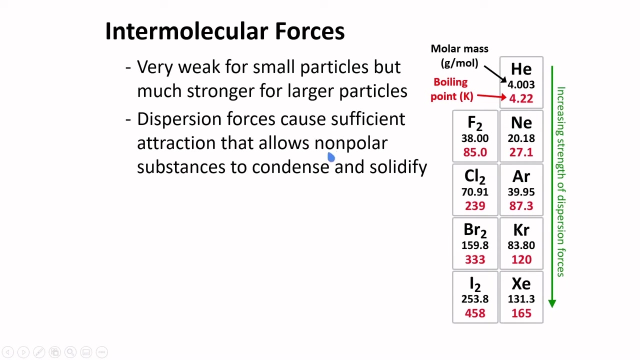 dispersion forces are very weak for small particles but are much stronger for larger particles. if we compare the noble gases, there's a general increase in boiling points as their size increases. this can be attributed to the increasing strength of dispersion forces. dispersion forces cause sufficient attraction that allows non-polar 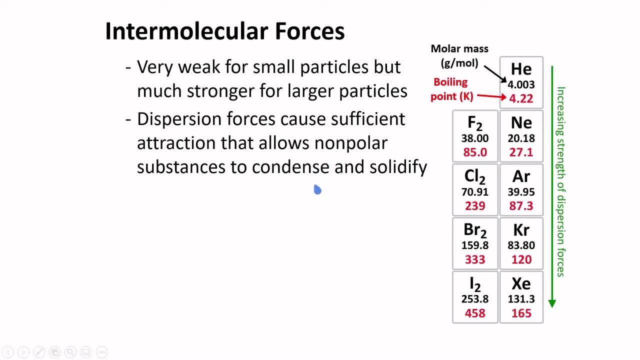 substances to condense and solidify. exane is a non-polar substance and yet it is liquid at room temperature. they contribute to the overall energy of attraction of all substances. they contribute to the overall energy of attraction of all substances. in hcl, 85 percent of the total energy of attraction is due to dispersion forces. 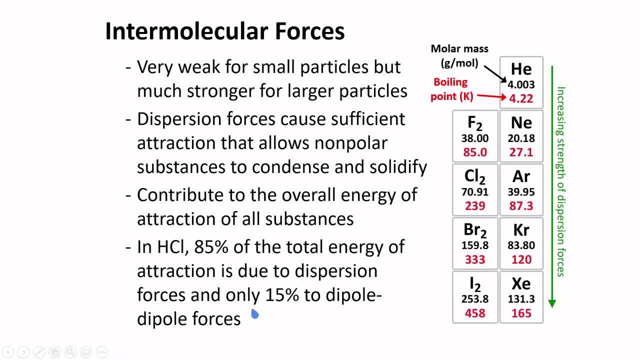 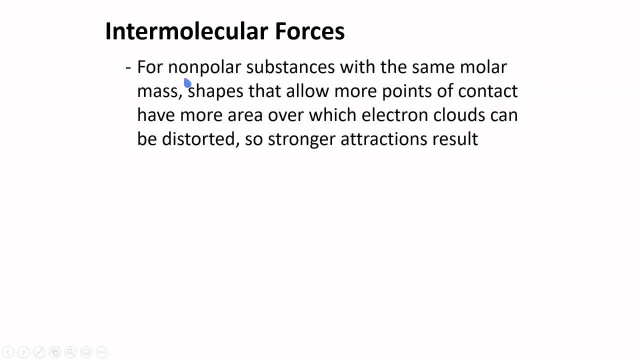 and only 15 percent due to dipole-dipole forces for non-polar substances with the same molar mass. shapes that allow more points of contact have more area over which electron clouds can be distorted, so stronger attractions result. in the case here for pentane, there are more points of contact for dispersion forces to act. 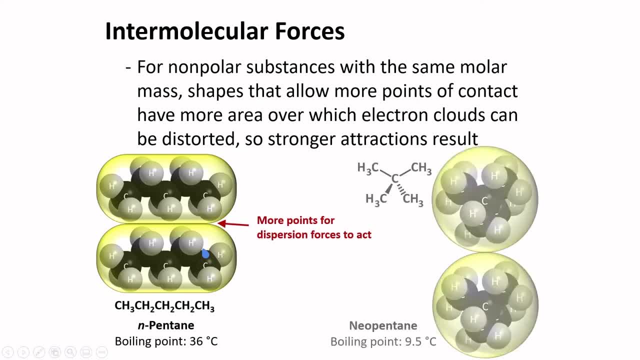 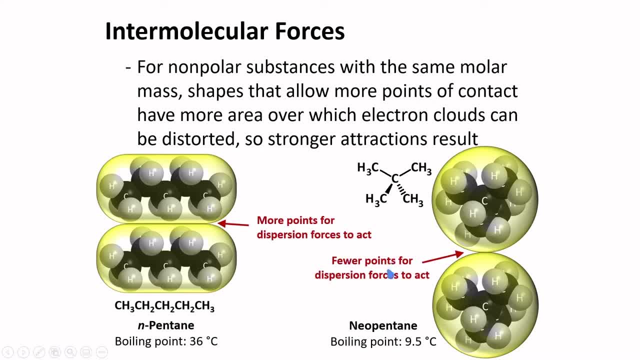 the shape of neopentane allows for fewer points for dispersion forces to act. hence the boiling point of neopentane is only 9.5 degrees celsius, despite having the same molar mass as pentane. in summary, we have ion dipole forces. 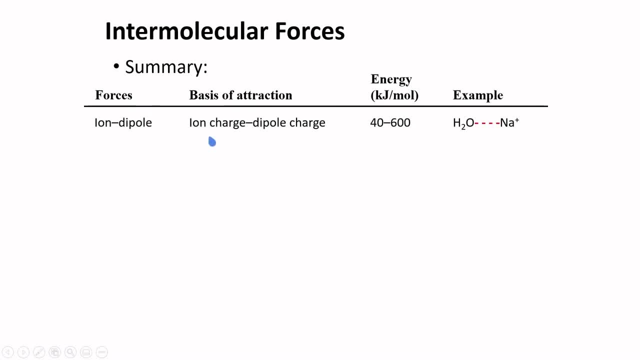 this is based on ionic charge and dipole charge, hydrogen bonding- this of course, in polar bonds to hydrogen- and the dipole charge. we have dipole dipole. there's ion-induced airport beeping dipole, where the ion charge of neopentane is no longer tired land. 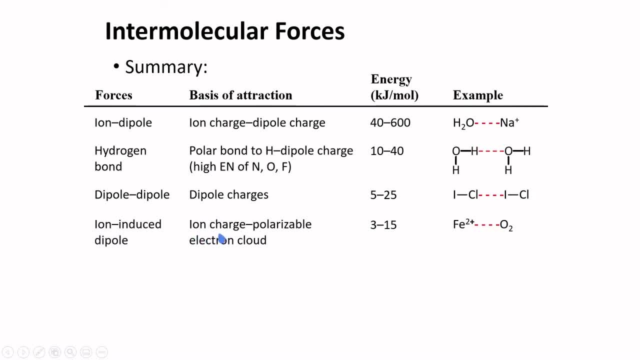 because implexic dipole has an alcohol-ool type dipole vitamin is attracted to a polarizable electron cloud. we have dipole induced dipole where a dipole charge is attracted to a polarizable electron cloud and dispersion forces the attraction between polarizable electron clouds. the trends in energy usually decreases in the order shown. 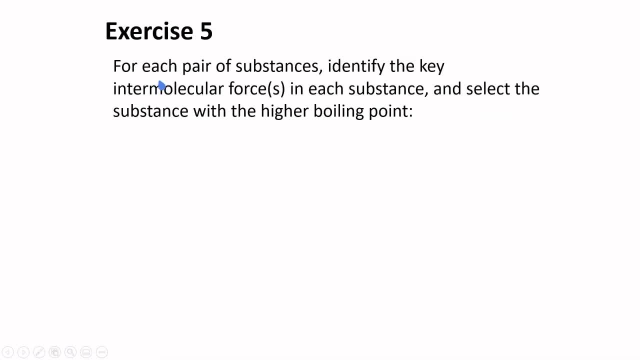 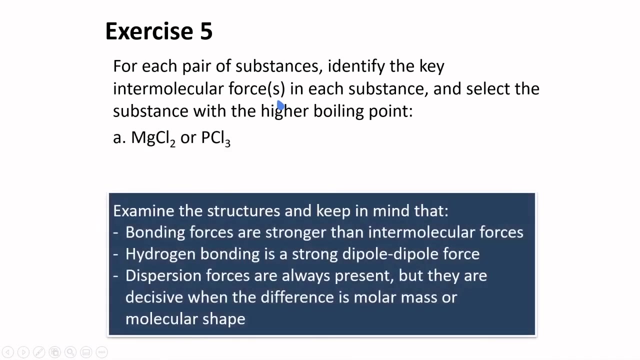 exercise 5 for each pair of substances. identify the key intermolecular forces in each substance and select the substance with higher boiling point better a magnesium chloride or phosphorus trichloride between. chloride is unable ionic substance, whereas phosphorus trichloride is a compound with molecules attracted to. 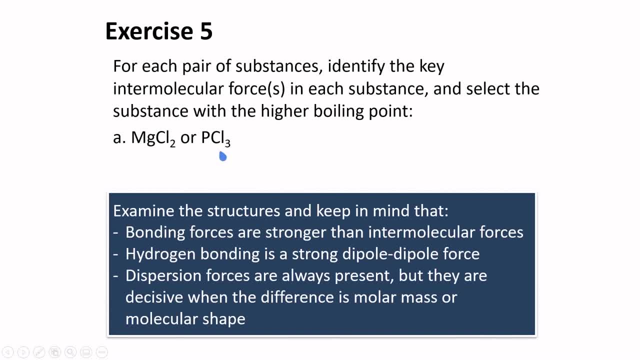 each other by van der Waals forces. Here you can expect that magnesium chloride has a higher boiling point compared to phosphorus trichloride by virtue of its ion-ion interaction, Methylamine or methyl fluoride. Hydrogen bonding can occur in methylamine, but not in methyl fluoride, where dipole-dipole forces can be expected. Hence the boiling point of methylamine should be higher. Methanol and ethanol: Methanol and ethanol- Both methanol and ethanol- exhibit hydrogen bonding. However, ethanol is a bigger molecule. and has a higher tendency for dispersion forces to act. Hence you can expect that ethanol has a higher boiling point than methanol Hexane: Hexane is a linear molecule, whereas 2,2-dimethylbutane is a bit spherical. There are more chances. 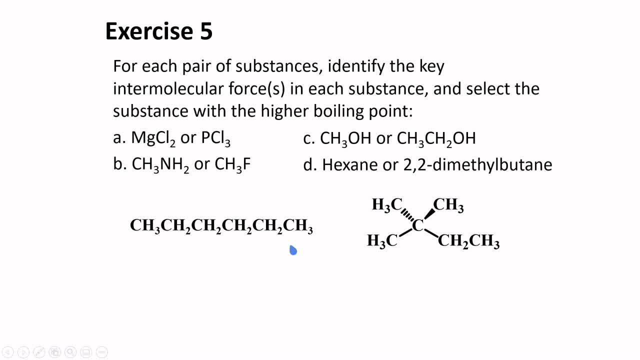 for dispersion forces to act for a linear molecule. Hence hexane should have a higher boiling point. Hexane is a linear molecule, whereas 2,2-dimethylbutane is a bit spherical. There are more chances for dispersion forces to act for a linear molecule.